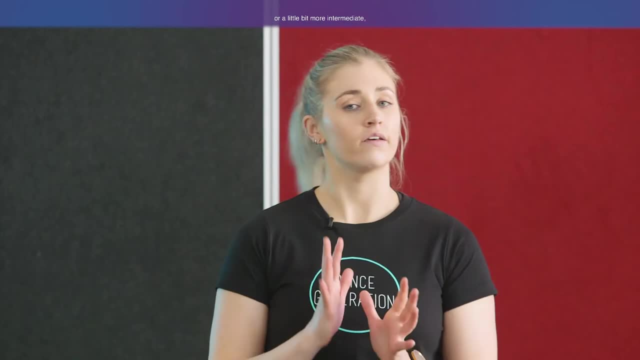 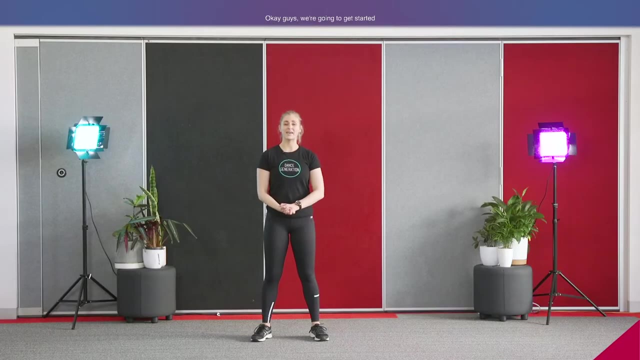 9 to 12. but if you're a beginner or a little bit more intermediate, you can kind of just make the dance a little bit your own, okay. Okay, guys, we're going to get started with a little bit of a warm-up, So let's bring our feet out so they're a little bit wider than our hips From. 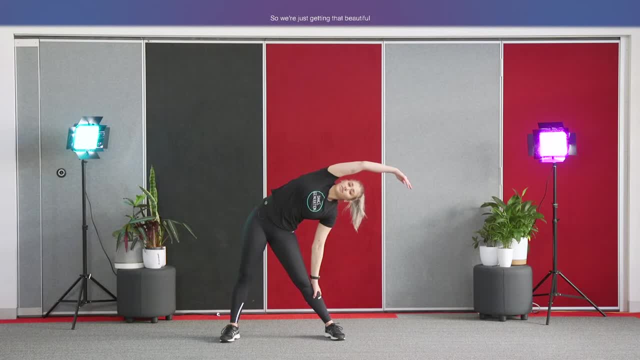 here, right arm reaches up and over. We're going to stretch through our sides. so we're just getting that beautiful lateral side body stretch, just lengthening through your side, reaching through the hands and out the energy with the opposite hip, getting that lovely long stretch. and then 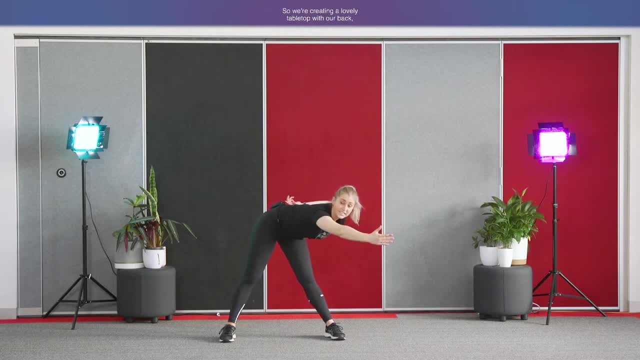 we're going to come through to a flat back position here. So we're creating a lovely tabletop with our back, reaching through the hand and then reaching back through the hip. So we're really elongating through the hand, getting that nice long stretch and all the way down to the leg. So let's let the 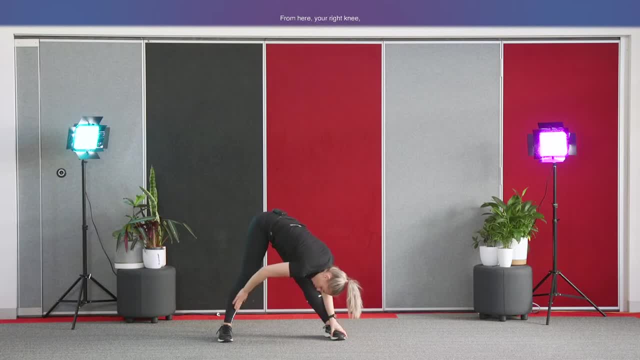 feeling that lovely stretch down the back of the leg From here your right knee so your opposite leg, is going to bend and stretch, bend and stretch. Are you guys starting to feel a little bit warm? I'm starting to warm up, feeling my muscles come alive. Four more here. four three, last two. 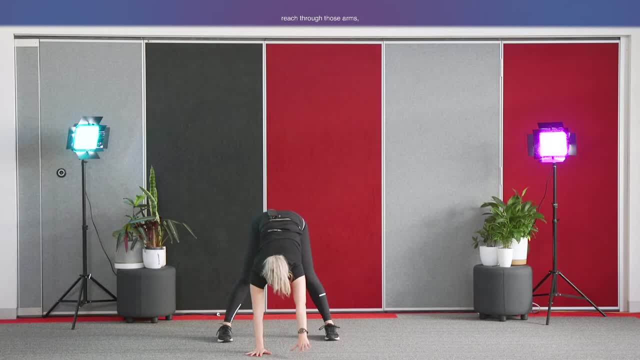 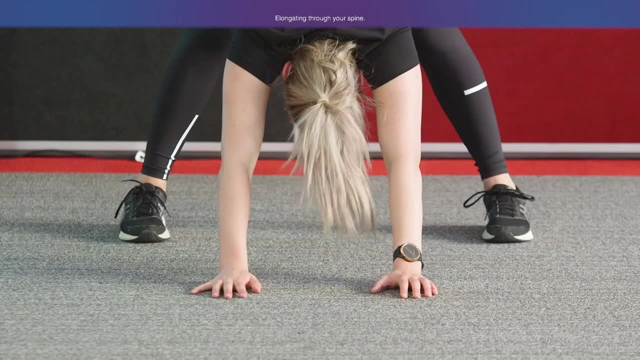 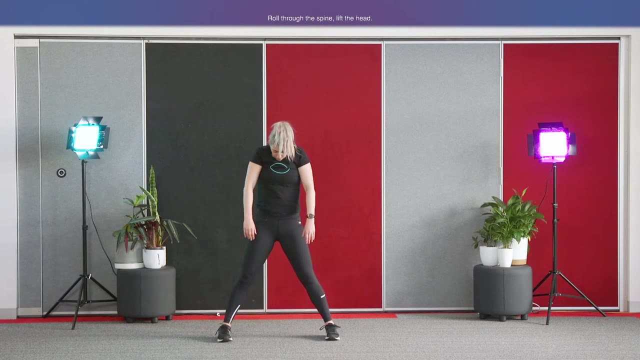 last one. Bring your hands into centre, reach through those arms, let your head drop and just really feel that lovely stretch Stretch through your back, elongating through your spine and rolling through and up right through the shoulders. Roll through the spine, lift the head, and other side Left arm reaches up and over. 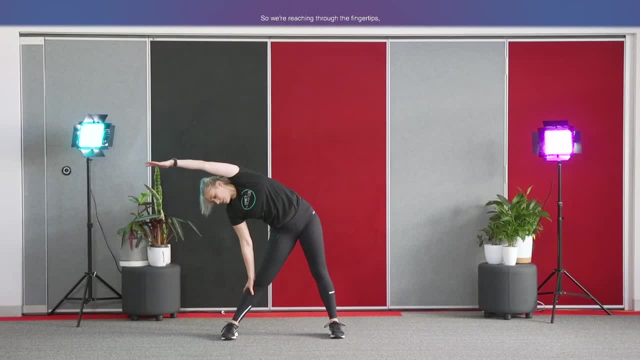 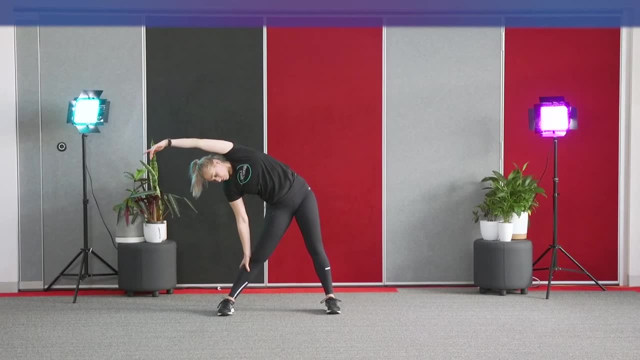 getting that beautiful side body stretch. So we're reaching through the fingertips and then reaching out through that opposite hip getting that lovely side body stretch, reaching, reaching, reaching and coming through to flat back. So we're reaching through that hand elongating. 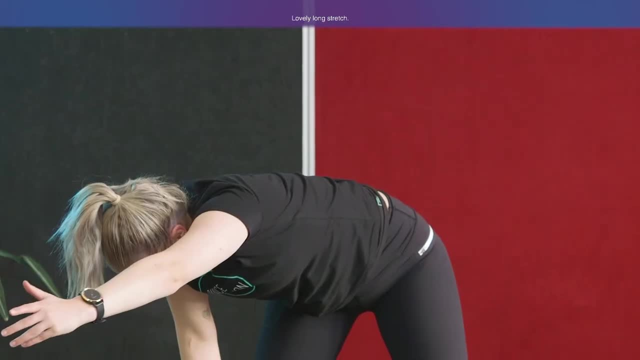 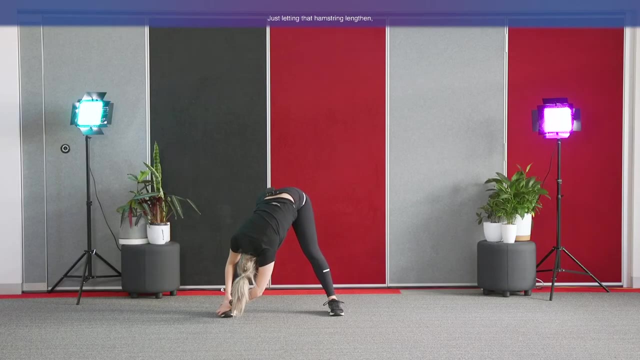 back through that hip- Lovely, long stretch, Beautiful. and then coming all the way down onto that leg. here, guys, Just letting that hamstring lengthen, stretching through your back- Nice, long stretch- and bending and stretching your left knee. So bending and stretching, bending and stretching. 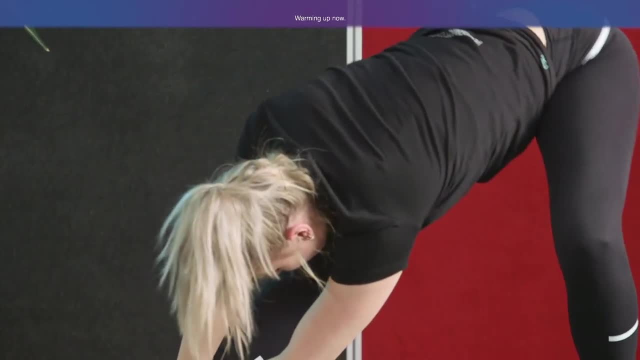 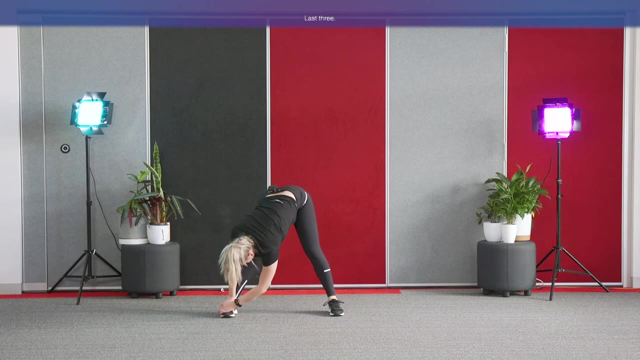 just getting that blood flowing through your body, Warming up. now Beautiful. Four more here to go: Last three, last two. last one: Bring your hands into centre, let your head drop, nice and heavy, elongating through your spine. Reach through those arms, getting that lovely long stretch. 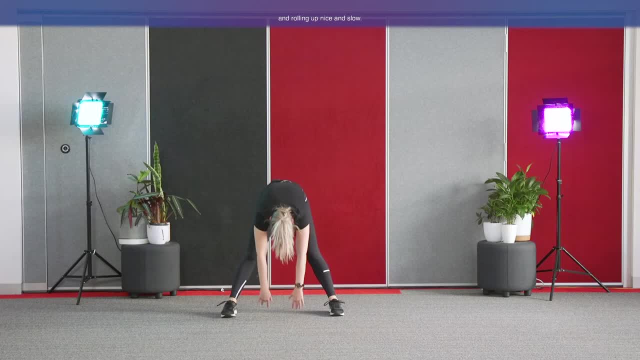 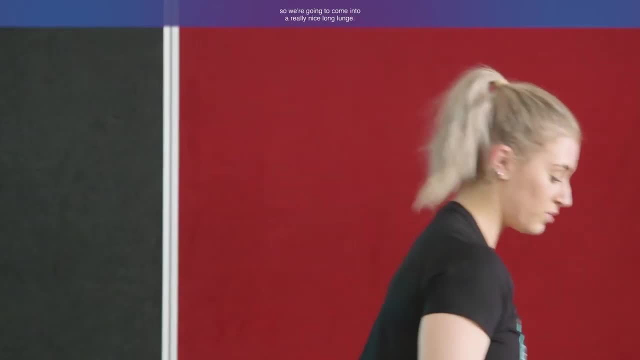 stretching down the backs of the legs and rolling up nice and slow Right through the shoulders and lift through the head- Beautiful. Let's turn side on now. We're going to go left leg forward, so we're going to come into a really nice long lunge, So we're opening up through that right hip. 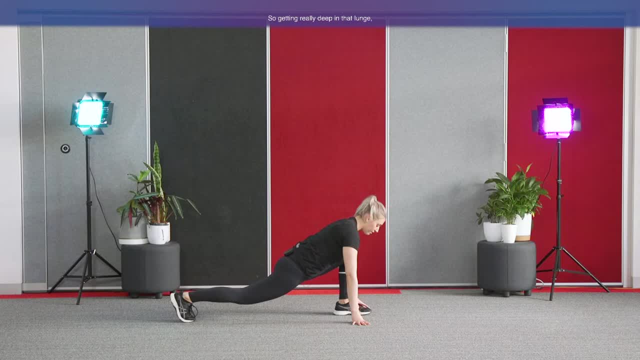 flexor here. So getting really deep in that lunge, stretching, stretching through that hip, Beautiful, Trying to straighten that back right leg, if you can, Good, and then we can drop that knee all the way down to the ground. We're going to kneel up nice and tall now, bringing both hands. 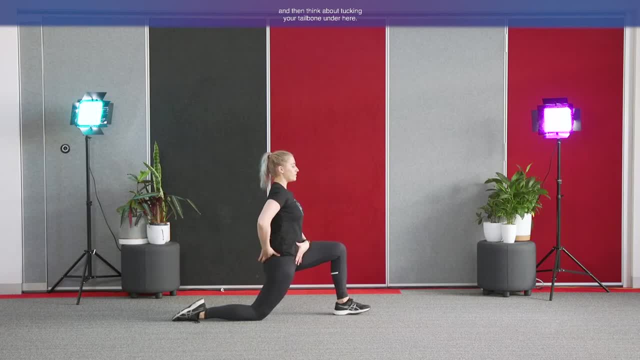 on that left knee and then think about tucking your tailbone under here. So we're tucking under and you should be feeling a really nice stretch down the front of that right hip. Good, Keep tucking, keep tucking and breathing. 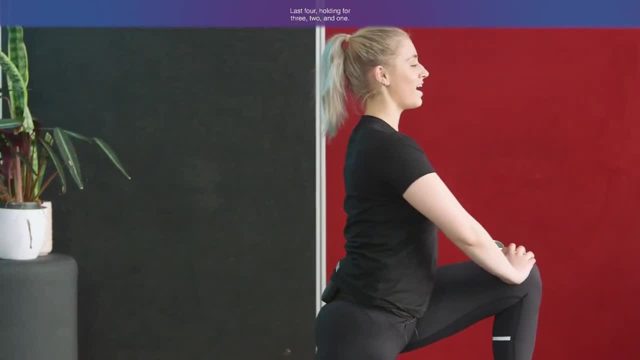 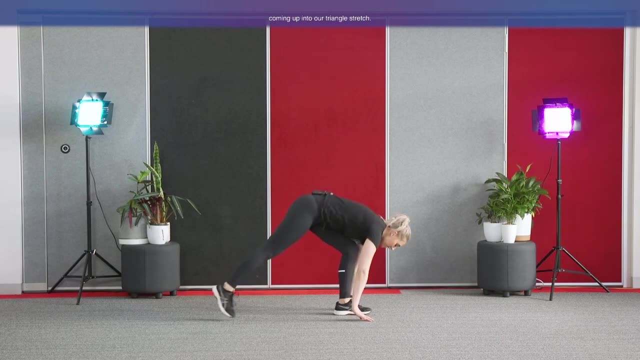 Shoulders always drawing down: Good Last four, holding for three, Two and one. Let's bring our hands down onto the floor, coming up into a triangle stretch, So stretching your head down towards that front. left leg, Two straight legs here. Hands are on either side of that front. 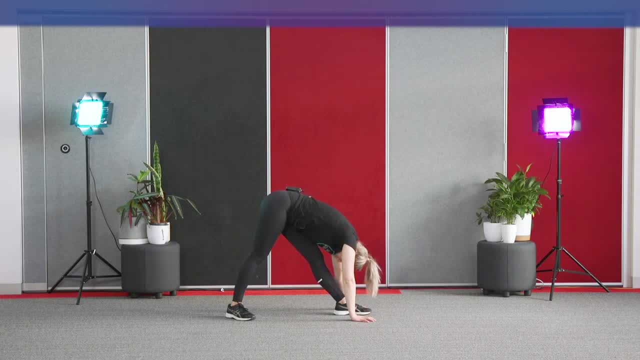 foot, getting that beautiful, lovely, long stretch, Lovely, lovely, And coming back down into your lunge one more time, Really, really good. And then we're going to come back down towards that front, opening through that right hip, getting that lovely stretch through that leg. and then let's turn and 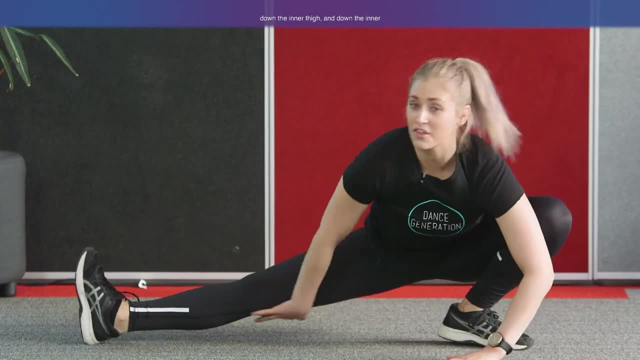 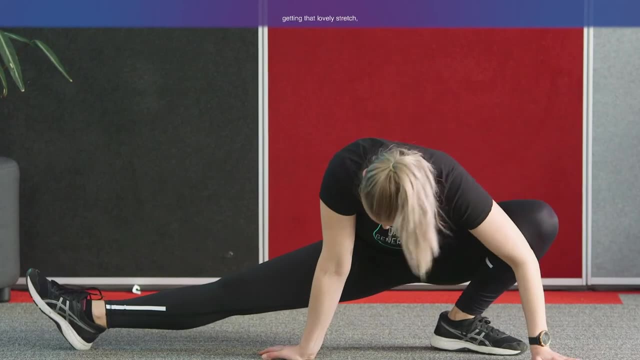 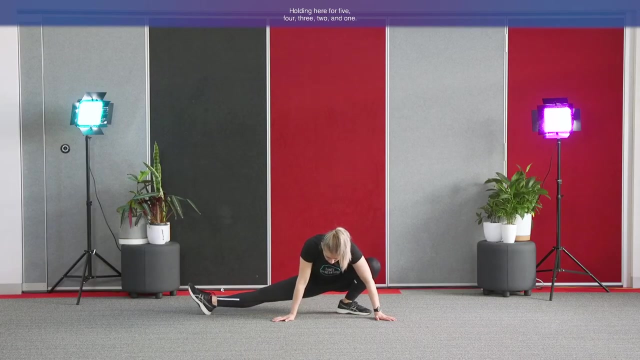 face forward. so we're going to get that beautiful stretch down the inner thigh and down the inner of that right leg, so always trying to turn those knees out, getting that lovely stretch, really just feeling everything warming up nicely, holding here for five, four, three, two and one. let's crawl over. 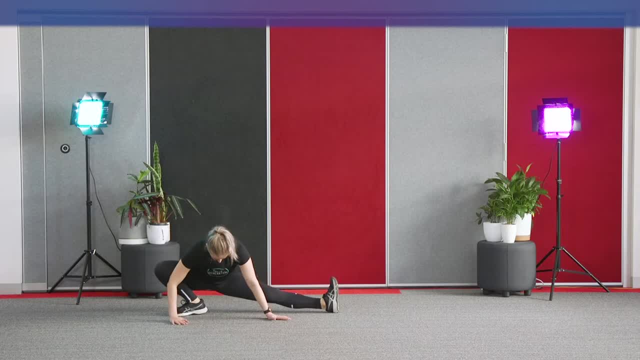 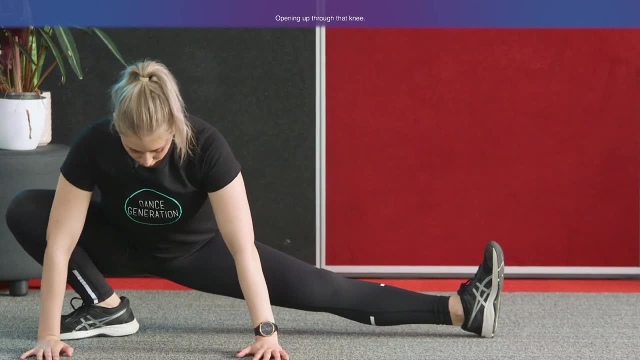 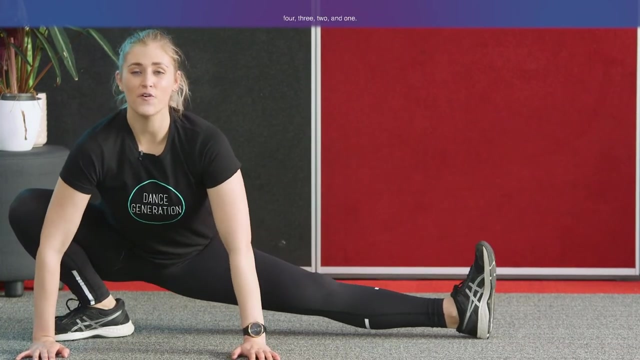 to the other side and stretch out the opposite hip, so really just feeling that lovely stretch down that inner thigh here all the way down to the ankle opening up through that knee. beautiful stretch here, lovely holding for another five, four, three, two and one. let's turn sideways. 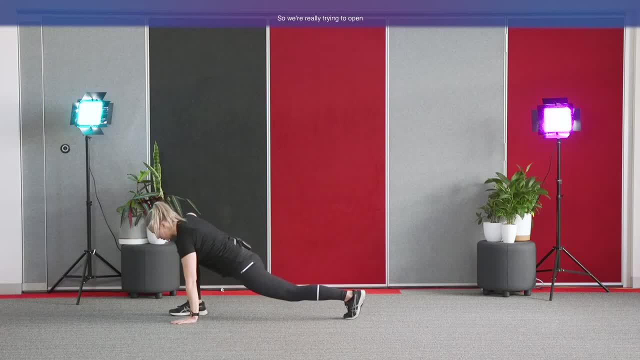 so coming into that beautiful lunge position here. so we're really trying to open and lengthen through the front of that left hip. now, guys, getting that beautiful stretch down that inner thigh here all the way down to the ankle, opening up through that knee stretch. good, keep holding, keep breathing. holding for five, four, three, two, one, pop that knee down. 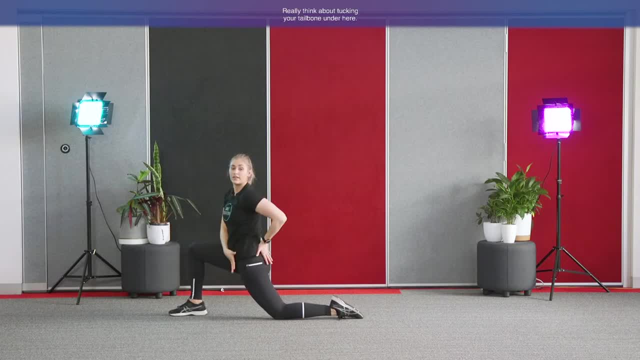 onto the ground. let's go both hands onto that front right knee. really think about tucking your tailbone under here, so you're getting that lovely, delicious stretch down through the front of that left hip and maybe down through that quad a little bit here. keep thinking about tucking. 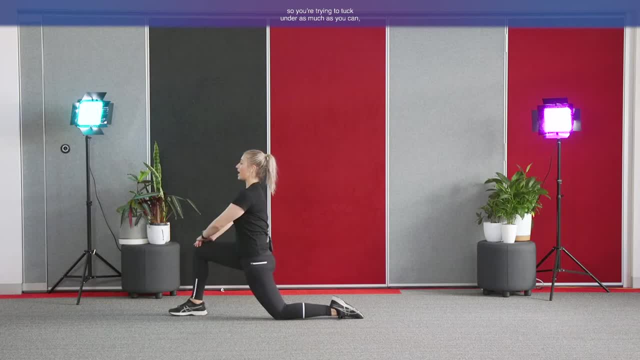 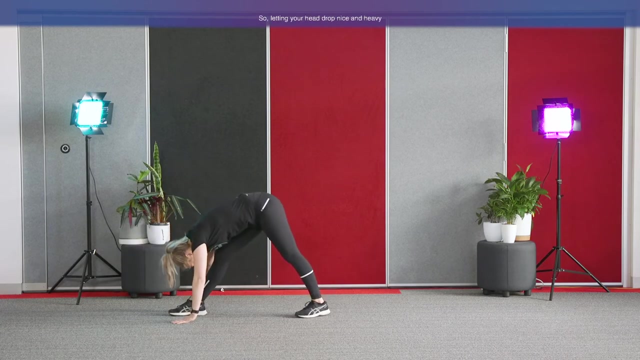 your tailbone under. so you're trying to tuck under as much as you can, maintaining that tuck, and that's really going to stretch through the front of that left side, holding for five, four, three, two and one, coming back up into our triangle stretch. so letting. 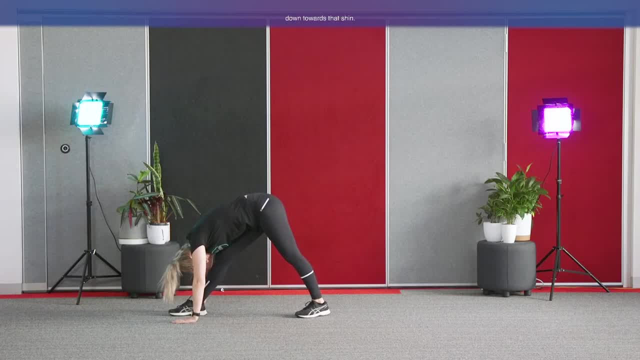 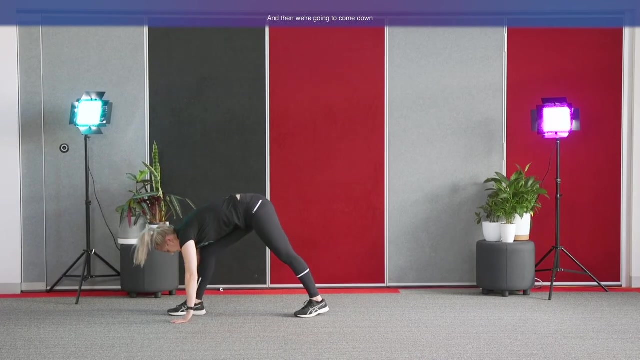 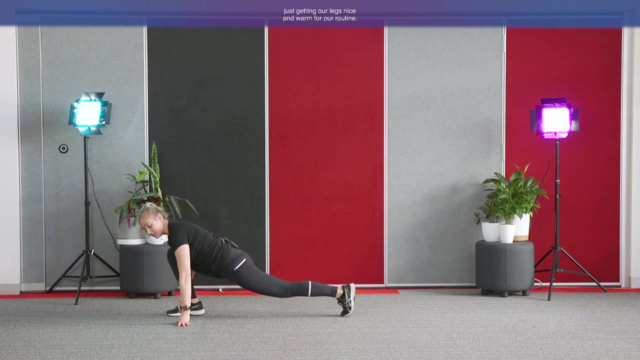 your head, drop nice and heavy down towards that shin- lovely. stretch down either side of the backs of the legs- beautiful work here, guys, really nice, stretch, lovely. and then we're going to come down to our lunge position one more time, opening through that left hip here, just getting our legs nice and warm for our routine. 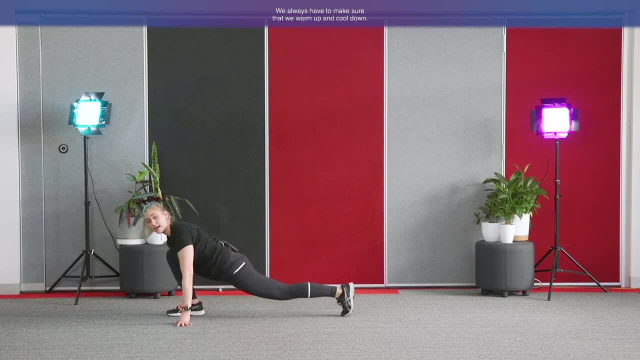 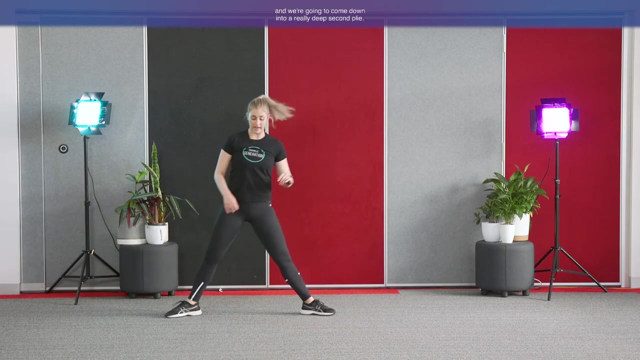 we always have to make sure that we warm up and cool down very, very important. we don't ever want to get injured. it's very important that we always properly warm up and cool down. okay, coming back up again, we're going to come to center this time. i want you to turn your toes out. 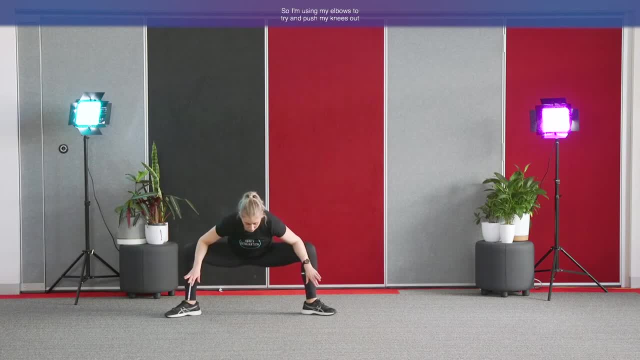 and we're going to come down into a really deep second plie. so i'm using my elbows to try and push my knees out a little bit more, so i'm really getting that lovely hip stretch here. so, through the hips and through the glutes, stretching, stretching, stretching. lovely work, guys. i. 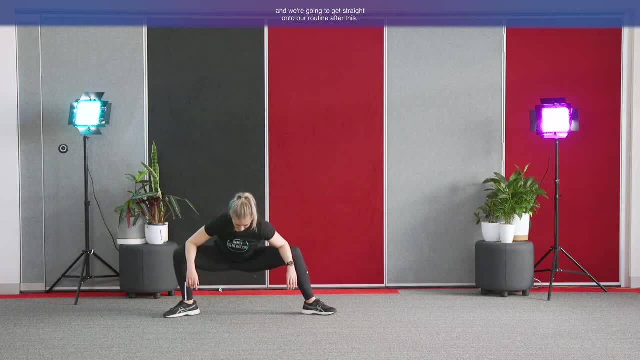 nearly finished warm up and we're going to get straight onto our routine. after this beautiful, let's turn the toes to face forwards. hands reach forward last time. let's turn the toes to face forwards, hands reach forward last time. your head drop nice and heavy, stretching through your back. 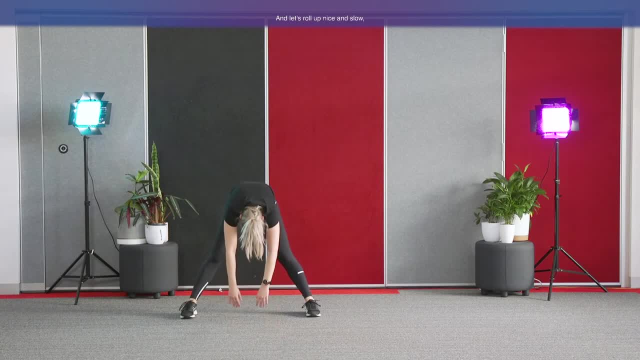 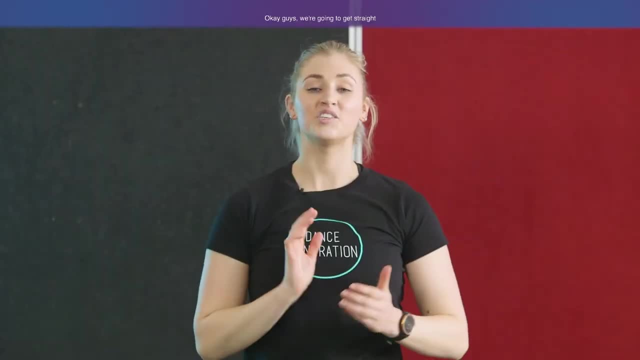 and let's roll up nice and slow, wrapping through the shoulders and lifting through the head. well done, guys. okay, guys, we're going to get straight into our dance routine now. so we're going to start knees and feet together like this and we're going to have that right knee popped. 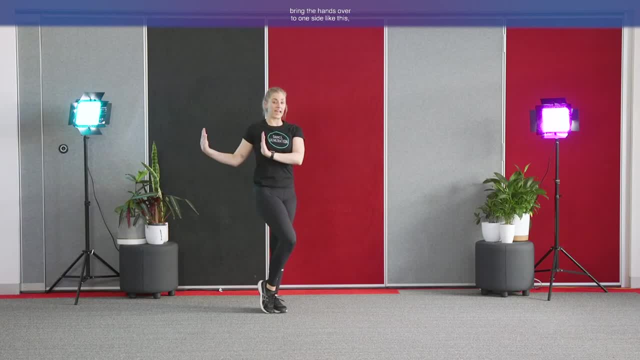 from here we're going to twist across to the side, bring the hands over to one side like this, and switch and switch and switch. so we're going to do that three times and then we're going to go ball change. so we're going to go right foot, left foot and we're coming into this turn. 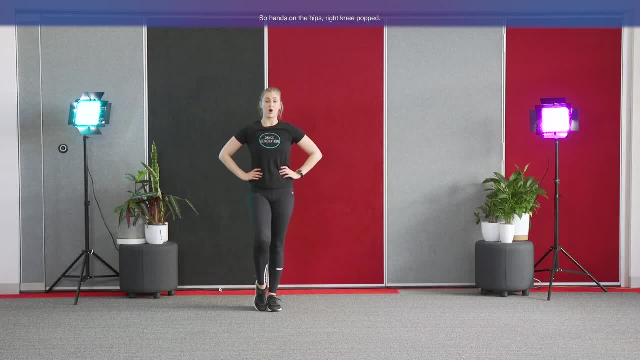 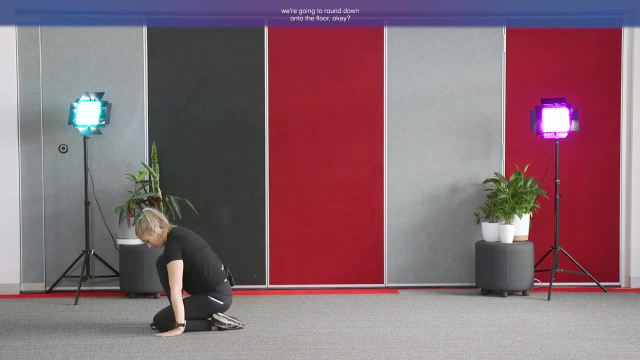 prep. let's do that again. so hands on the hips, right knee popped from here and a one and a two and a three and four into this turn position from here. one pirouette, so we're going to turn and then from here we're going to round down onto the floor. okay, let's do that again from the top. so 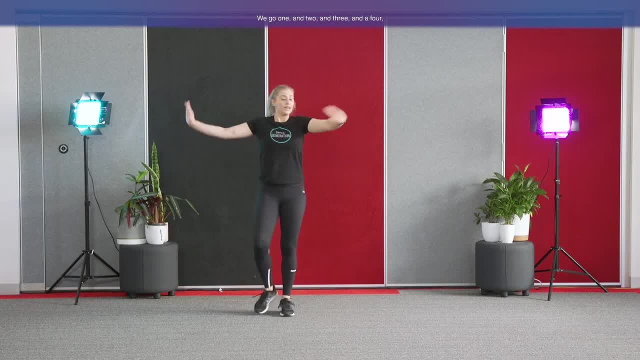 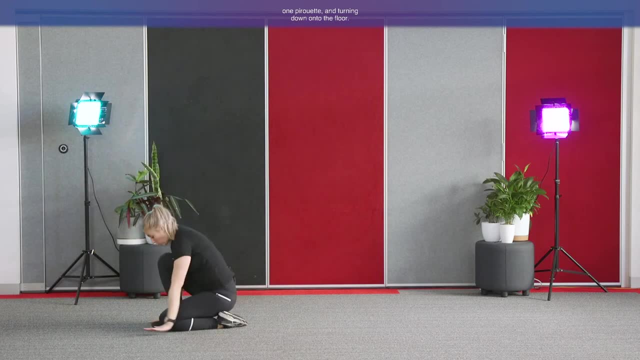 hands on your hips, right foot popped. we go one and two and three and four into this turn position. we go one and two and three and a four, one pirouette and turning down onto the floor. from here we're going to roll backwards, so rolling on your butt, rolling into this position where we have 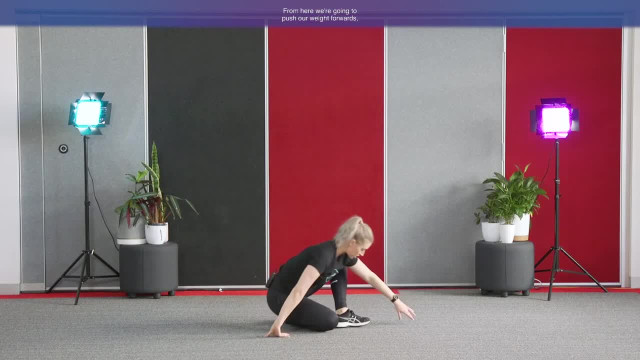 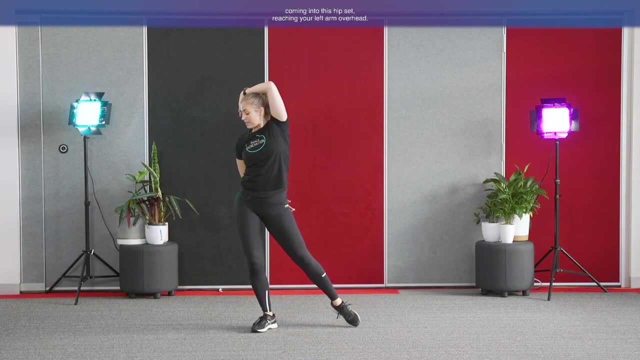 the right knee tucked and left foot up. from here we're going to push our weight forward and then we're going to come up into a little ponche and then we're going to swing the arms round, coming into this hip sit reaching your left arm overhead. let's go through that again, because i went through. 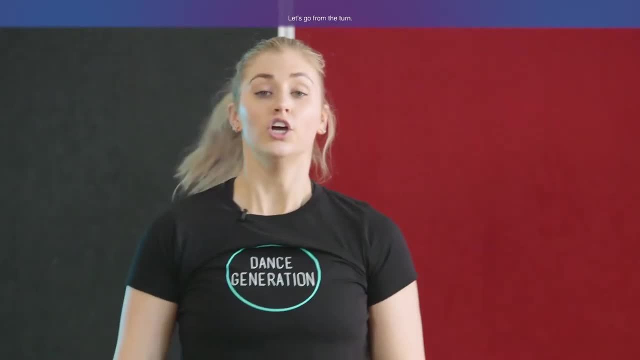 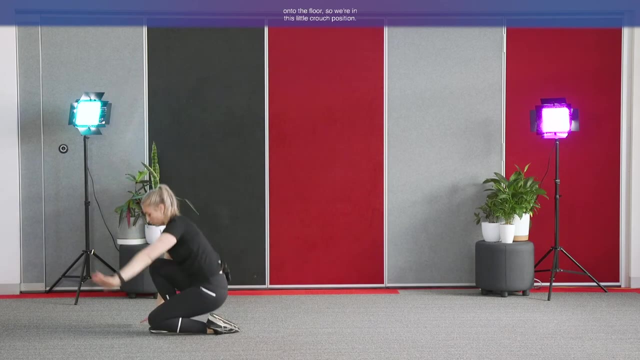 that quite quickly. let's go from the turn. so we go ball change from here pirouette, and then we go round and down onto the floor. so we're in this little crouch position. from the crouch position you're going to roll over onto that hip. hands go behind you rolling. so you've got that right knee. 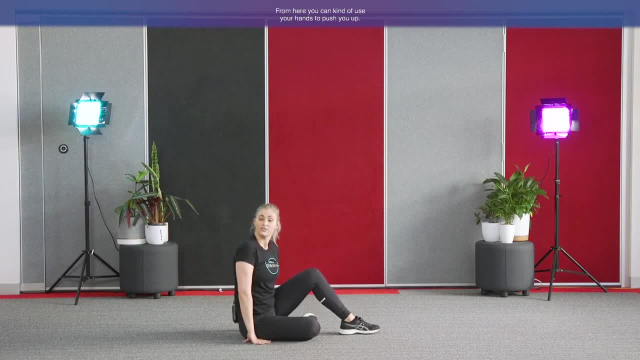 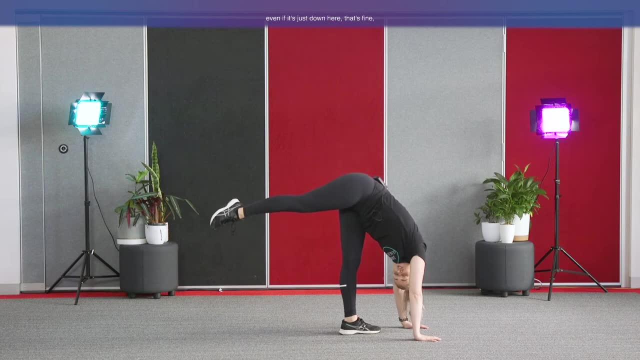 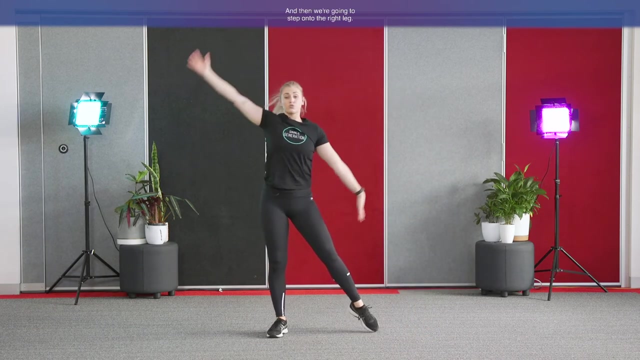 tucked up and left foot forwards. from here you can kind of use your hands to push you up. bring your hands down onto the floor and then we're going to go forward, and then we're going to go back and forth and then we're going to step onto the right leg, bring that left arm up overhead. so we're kind. 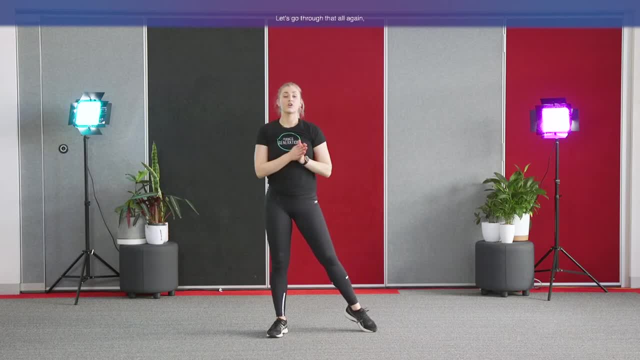 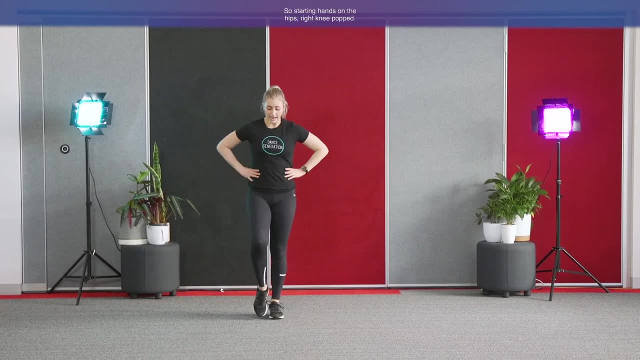 of coming into this little pose position. let's go through that all again one more time from the top, without the music, and then we'll try it with the music. it's quite fast, okay? so starting hands on the hips, right knee popped. from here we go one and two and three and four and five and six and seven. 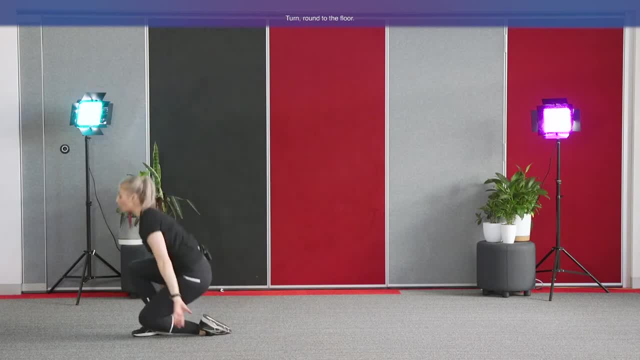 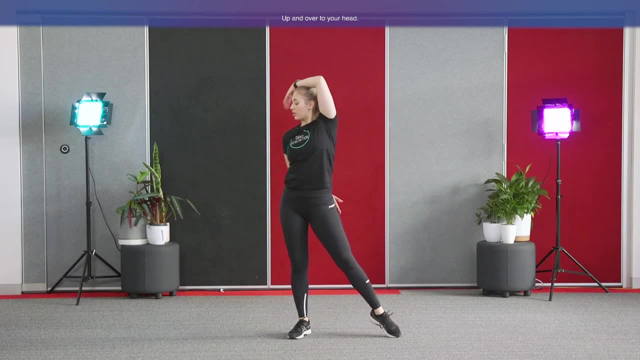 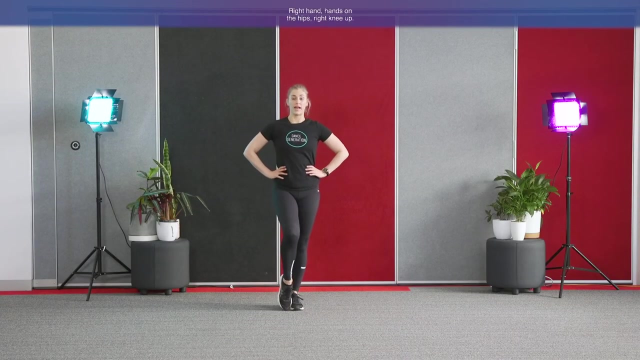 and a four turn round to the floor, roll from here. hands onto the floor, up and over to your head. okay, let's try that with the music. okay, guys, so we have a little bit of an intro. right hand our hands on the hip, right knee up. five, six, seven. we go one, two, three and four. five, six, seven, eight roll two. 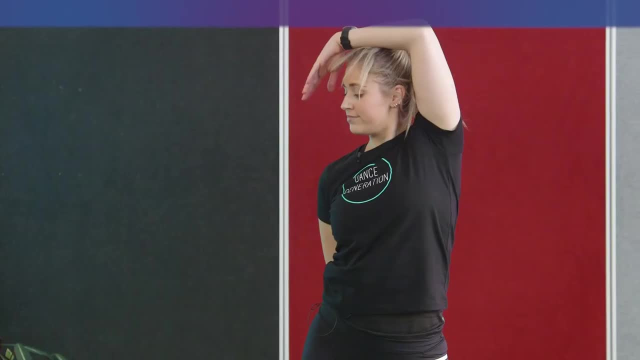 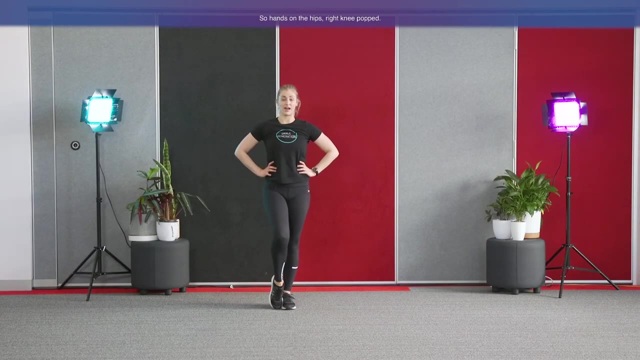 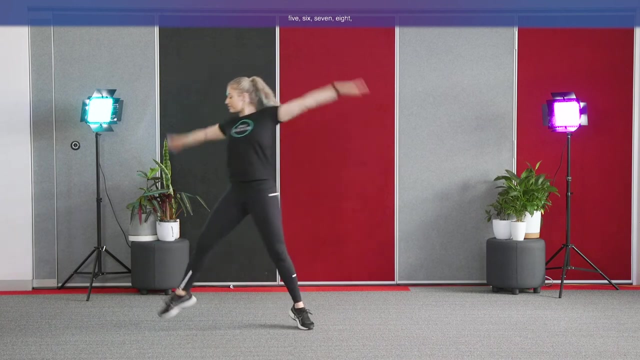 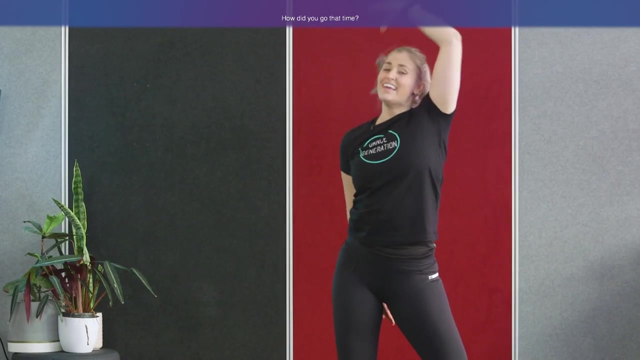 three, four leg over. did you get that? let's do that one more time. let's do that one more time, guys. so hands on the hips, right knee pops and five, six, seven and a one, two, three and four, five, six, seven, eight, one, two, three, four up over. how did you go that time? let's move on now. beautiful, thank you, music maestro. okay, so. 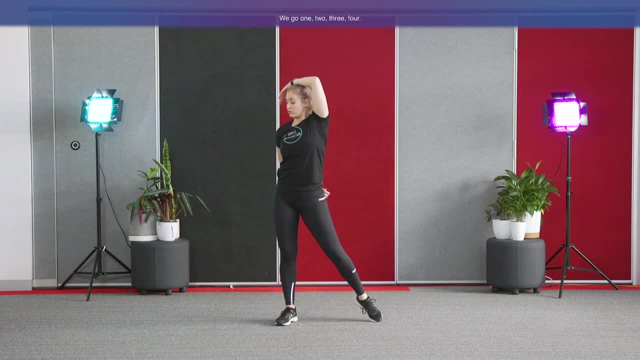 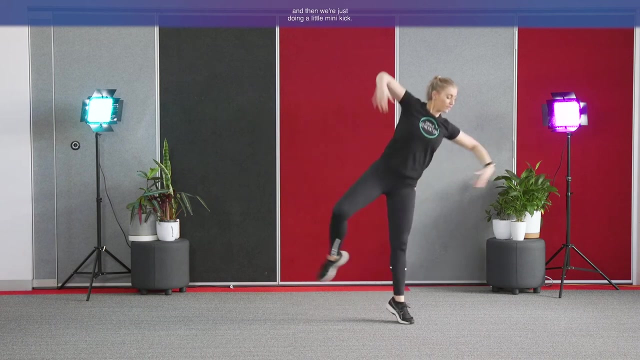 from here we go hand over the head. from here we do hip rolls. we go one, two, three, four. from here with our left leg we're going to draw a little in and out. so we're kind of drawing like a little zigzag with that left foot in, out, stepping onto that left foot, and then we're just doing a little mini kick. 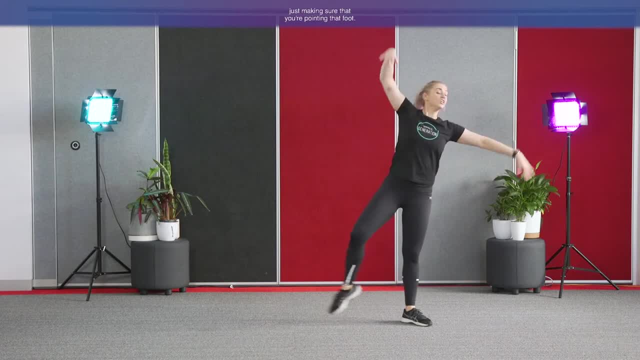 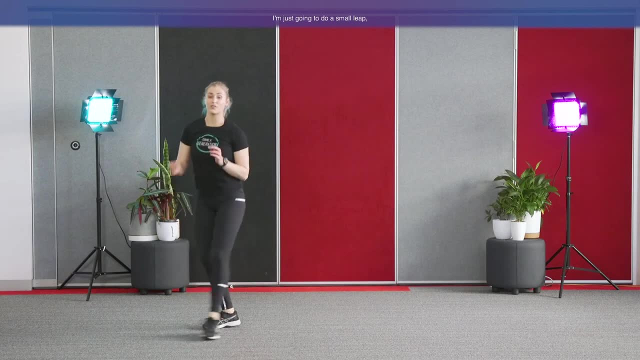 if you like, you can bring your leg all the way up, but if not, just a little one, just making sure that you're pointing that foot. so we go and up, step, step, leap. i'm just gonna do a small leap, because i small leap, because I don't have that much space, but you can do a really lovely big jeté if you. 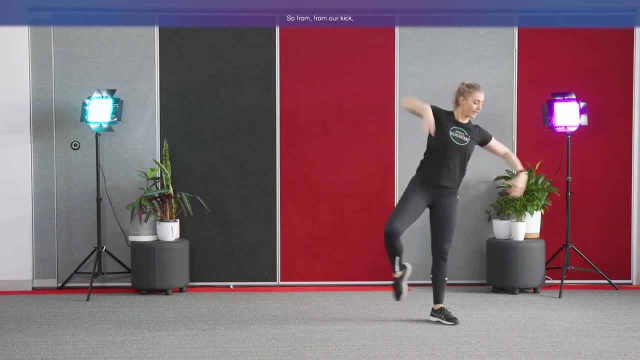 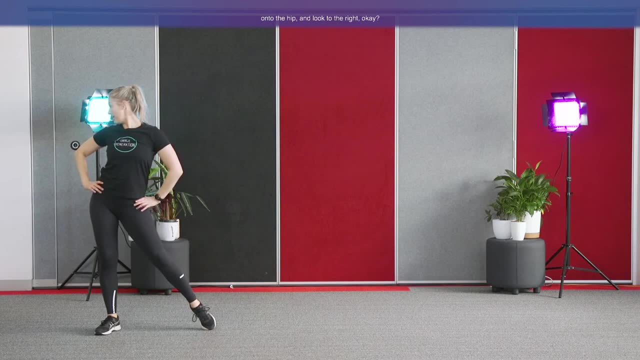 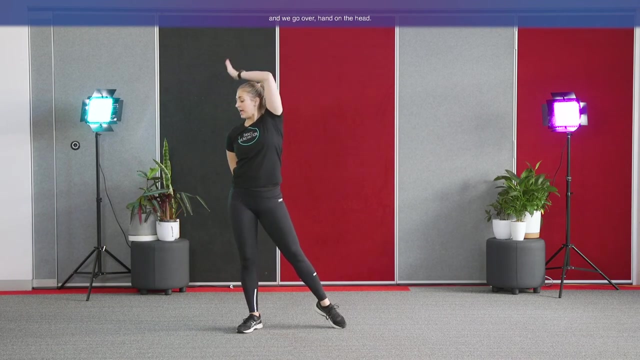 like so. from our kick we go step, step, leap, step, step onto the hip and look to the right. okay, let's go through that again. so we finish with the ponche and we go over hand on the head. from here we go one, two, three, four. little zigzag with that left foot zigzag in out step, bring the arms in. 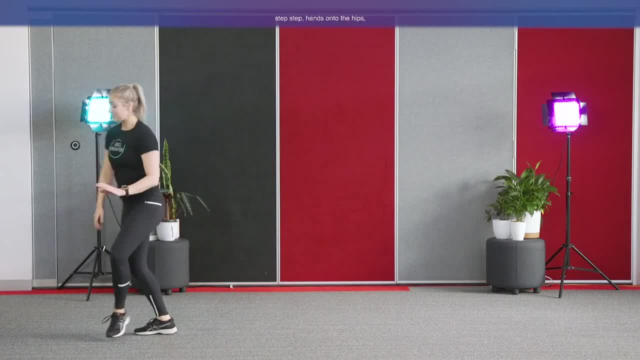 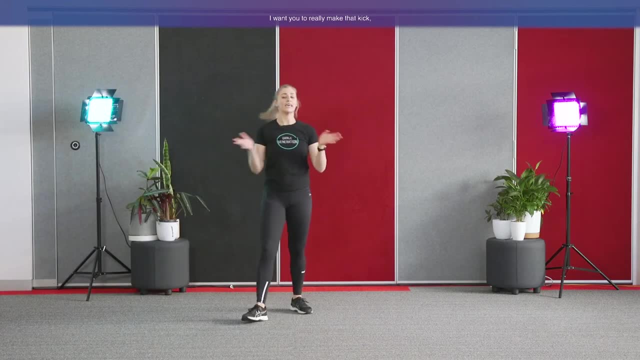 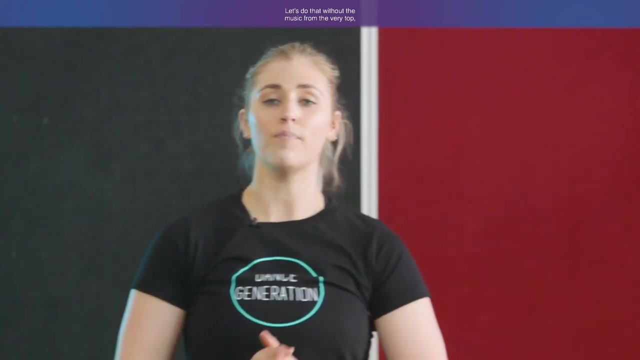 bring them up on the diagonal, step, step, jeté, step, step, hands onto the hips and look to the right. okay, if you've got more space than me, I want you to really make that kick and the jeté really lovely and big. okay, let's do that again. let's do that without the music, from the very top, and we'll. 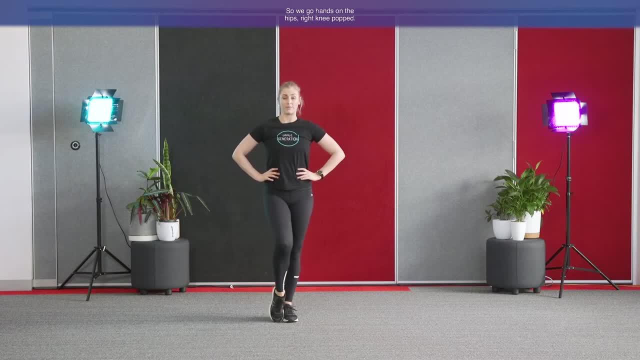 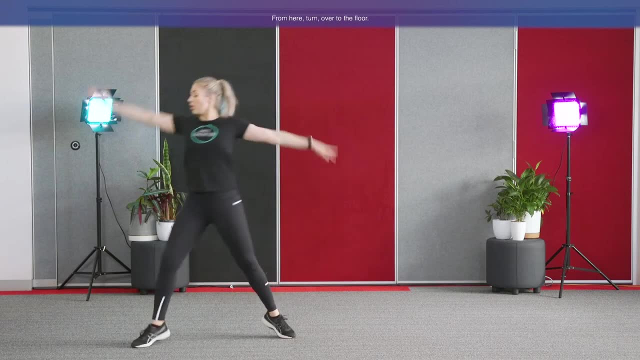 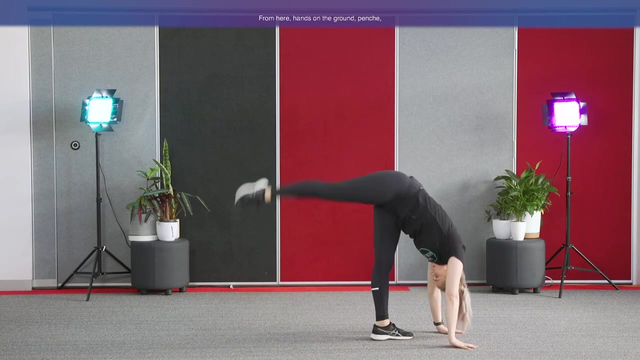 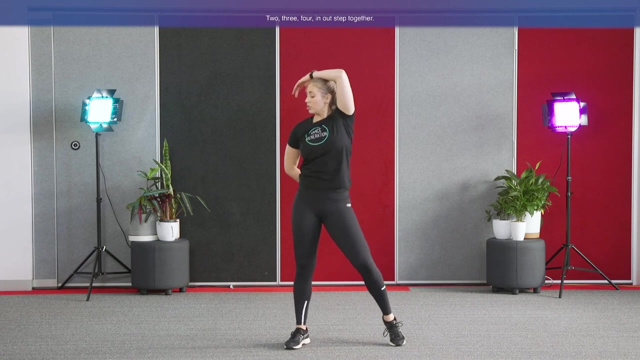 add that new bit on. so we go, hands on the hips, right knee popped, we go one and two, three and a four. from here turn over to the floor rolling onto your butt. from here, hands on the ground ponché, and we go over. bring the hands over to the head from here. hip roll, two, three, four in out, step together, little kick, step, step. 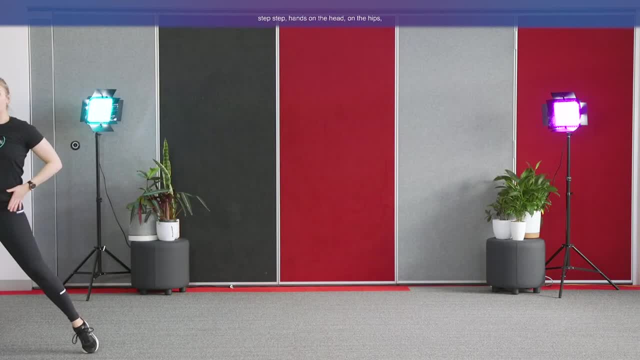 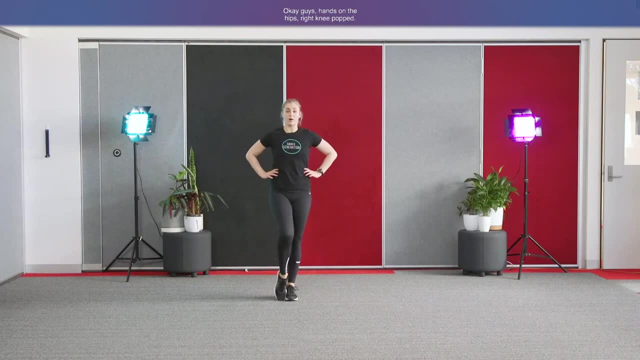 jeté, step, step. hands on the head, on the hips and look to the right. shall we try that again with music? okay, guys, hands on the hips, right knee popped, five, six, five, six, seven. we go: one, two, three and four, five, six, seven, eight roll two, three, four. 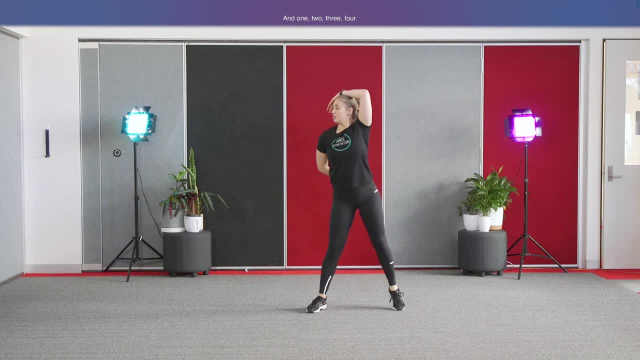 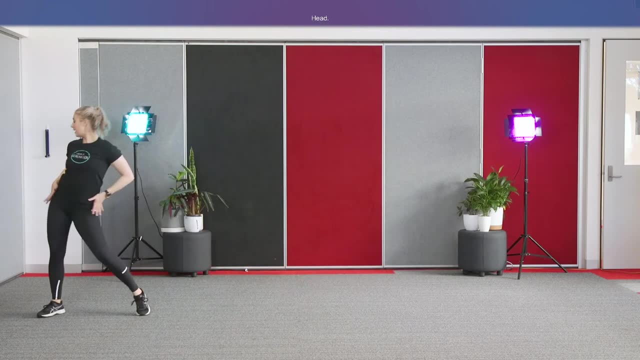 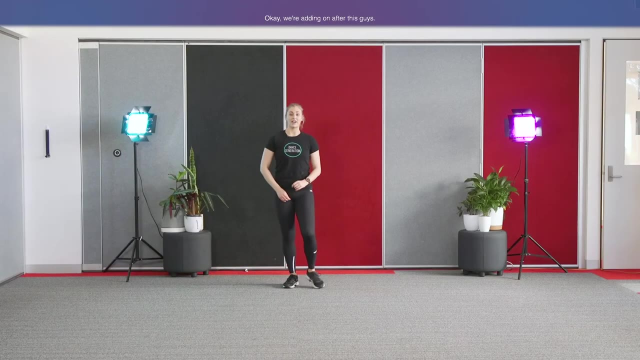 penche over, and one, two, three, four in step up, step, step, leap head. how did you go? let's do it one more time. okay, we're adding on after this guys. so hands on the hips, right knee, popped five, six, seven and a one, two, three and four, five. 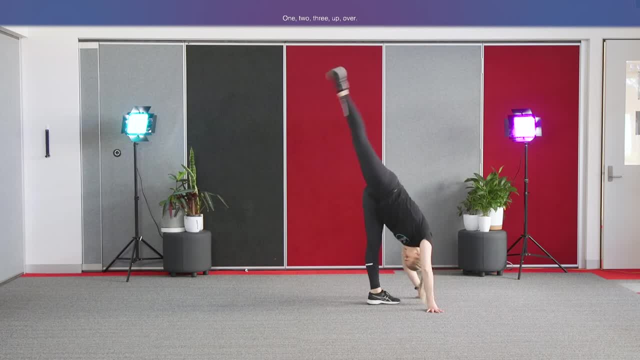 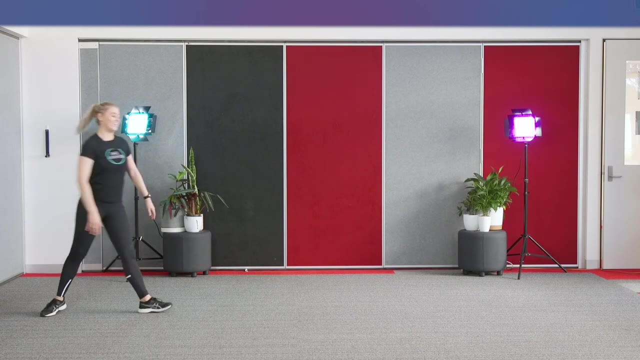 six, seven, eight, one, two, three up over and one, two, three, four in step, step, step, step, step, head. how did you go that time? it is quite quick, beautiful. let's add on now, guys. so we've just done the jet a and then we step over. we're looking to the right from here, back ball. 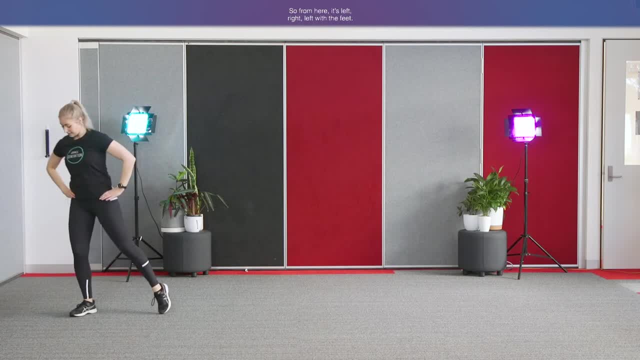 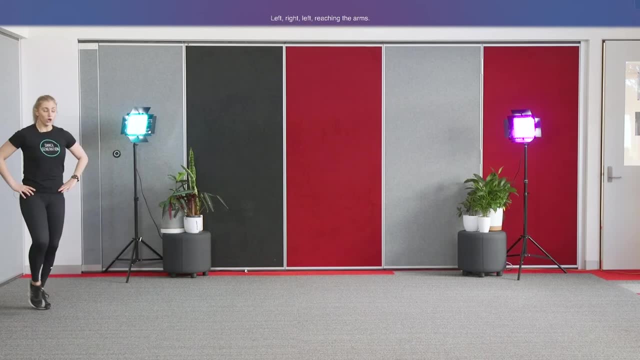 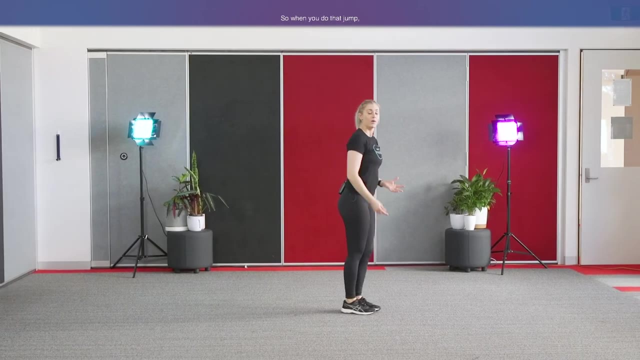 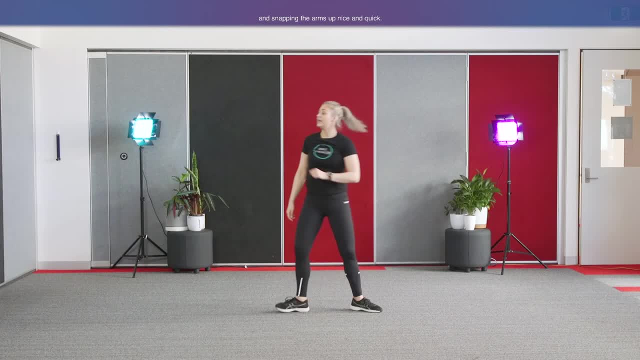 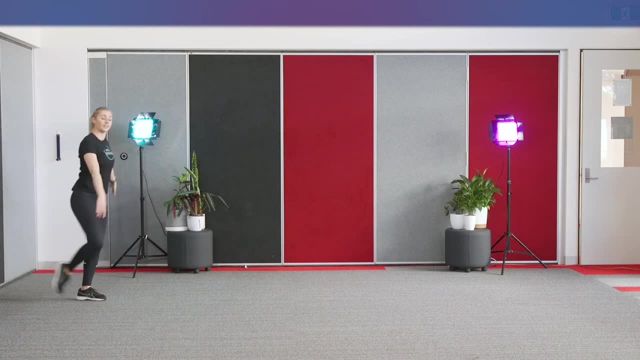 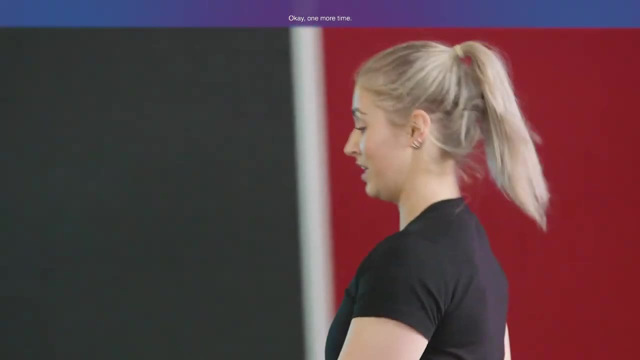 knees and feet together and snapping the arms up nice and quick. let's go through that again. so from here we go left, right, left, step, step, jump, step, step, step. okay, one more time. so from over here, we've got hands on the hips, head to the right. 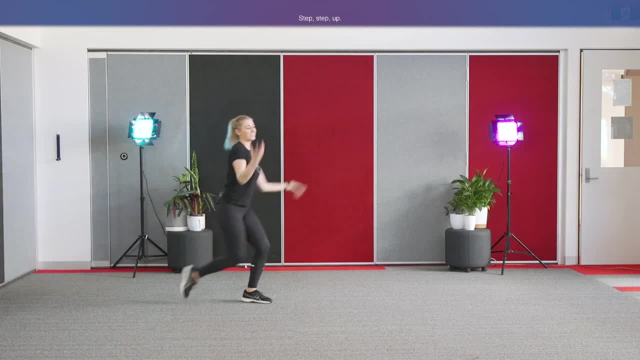 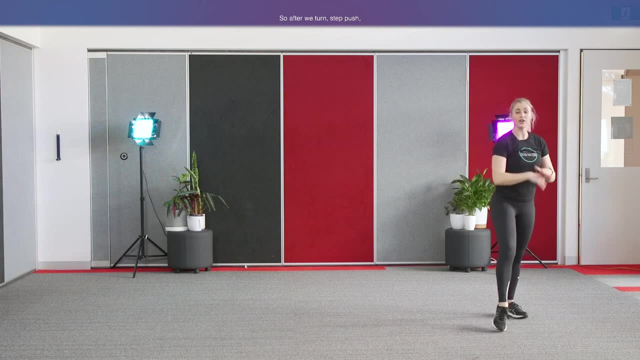 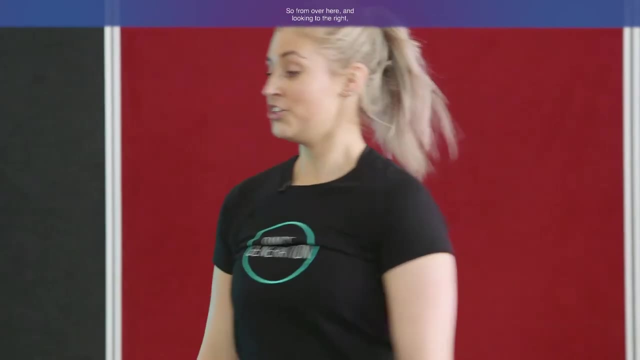 left, right, left left, step, step up, turn and turn. from here we're going to push to the front. so after we turn, step, push and then we walk back into the center of the room. okay, let's do that again. so, from over here and looking to the right, 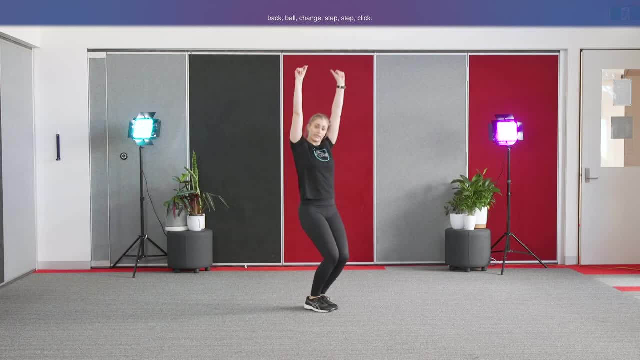 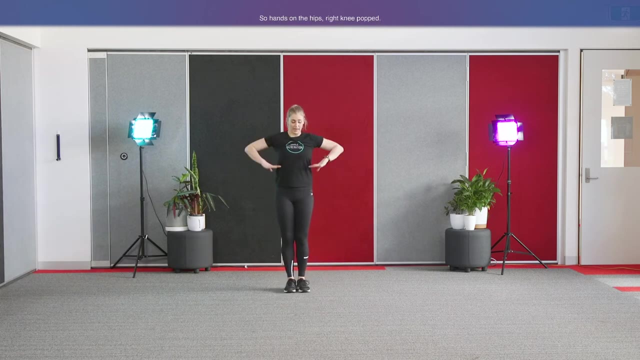 back ball change, step, step, click, turn and down, step push, and you're kind of walking on a little bit of a diagonal to the back. all right, let's put that together without music from the top, okay. so hands on the hips, right knee popped. from here we go one and two, three and a four, turn and around onto the floor. 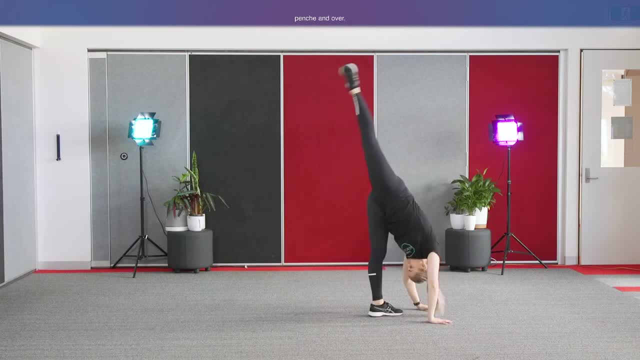 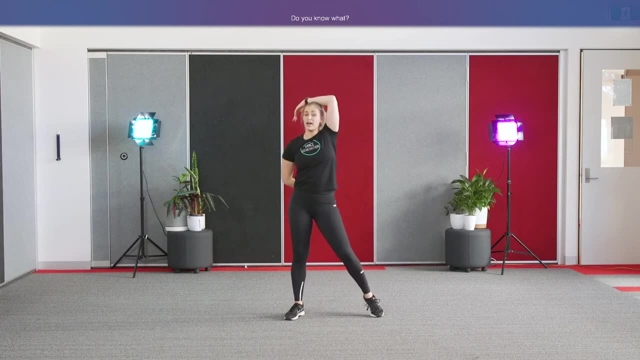 we're going to roll. push through the floor, the hands Ponche and over. That's the really fast bit. From here, roll two. Do you know what? I think it actually might work better if we only did three hips and not four, So let's do that. 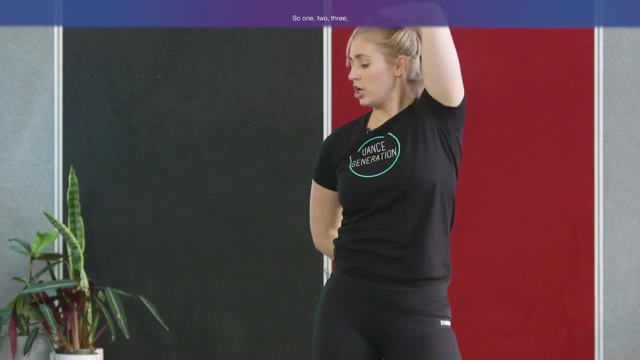 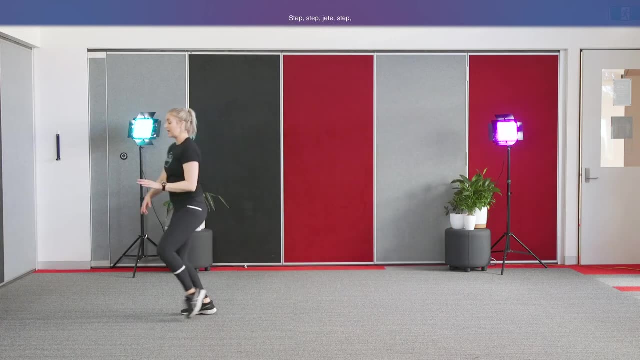 Just so we have a little bit more time to do the jeté. So one, two, three in out, step, kick, step, step, jeté, step and look towards the wall From here back ball change, step, step. 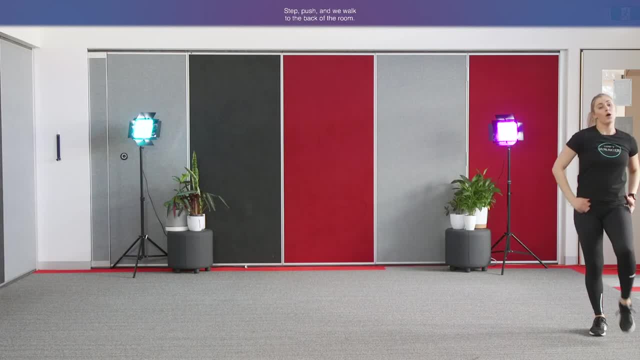 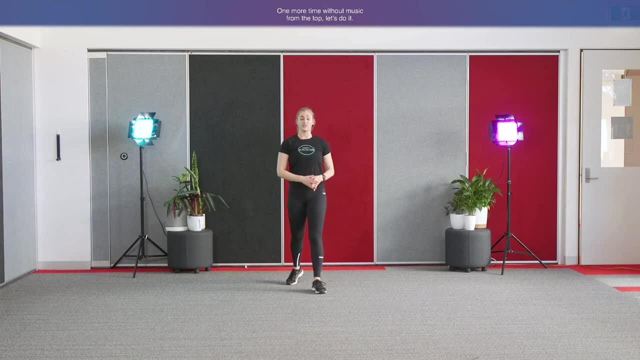 jump, turn and down, step, push and we walk to the back of the room One more time, without music from the top. Let's do it So, right knee, popped, hands on the hips, and we go one, two, three and 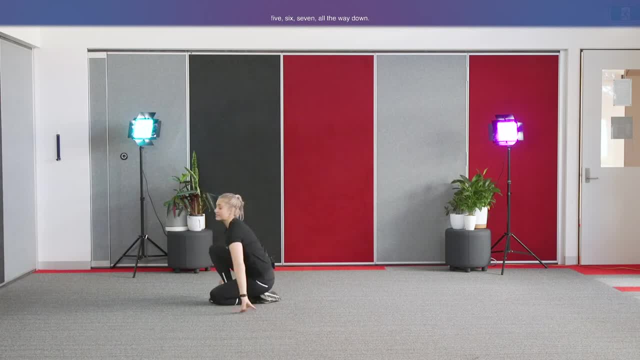 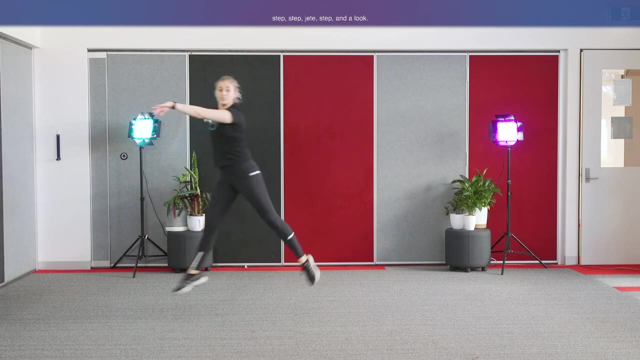 four, five, six, seven. all the way down, Roll two, three, four- even if it's a little one, and over to the head. Three hip rolls, not four, two, three and step up, step, step, jeté, step and look. one and two, three and four. 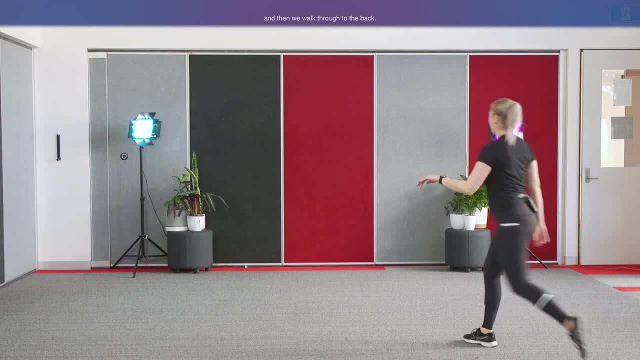 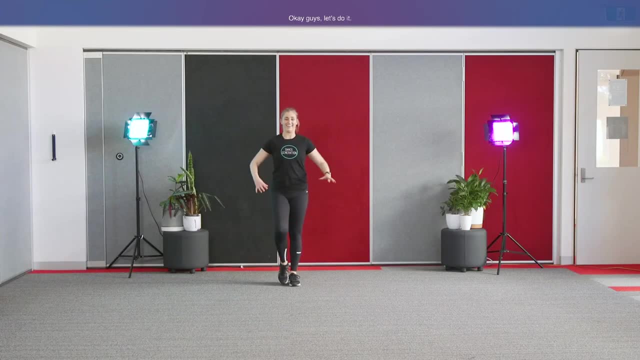 turn and down, step, push, and then we walk through to the back. Let's try it with the music. Okay, guys, let's do it. Ready, Five, six, five, six, seven, eight and a one two. 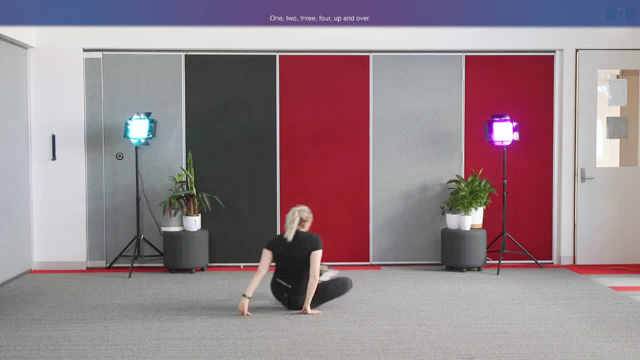 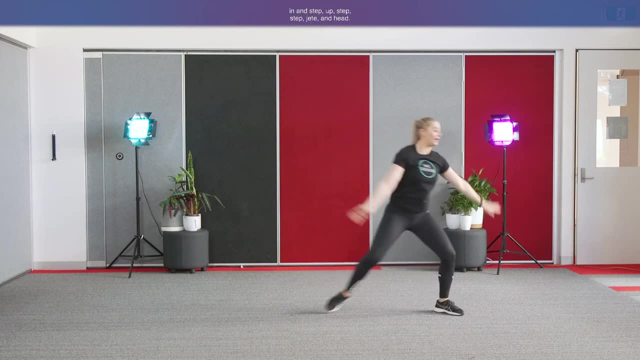 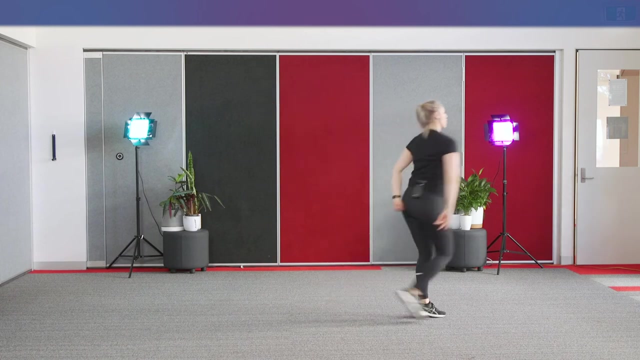 three and four, five, six, seven, eight, one, two, three, four up and over and hip two, three in and step up, step, step jeté and head Back ball change, step, step up turn. 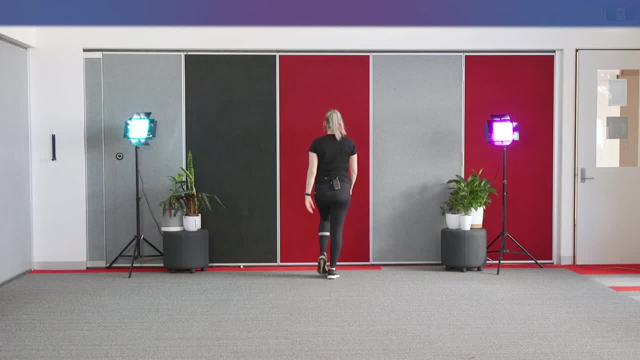 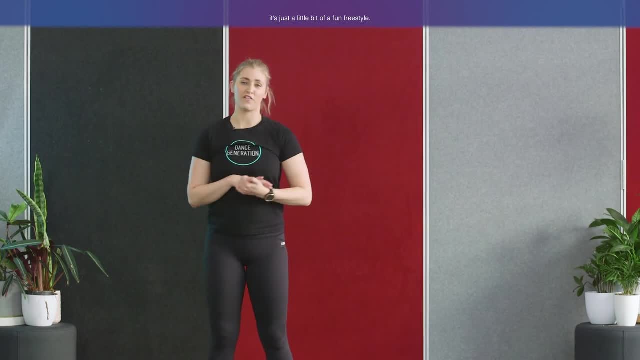 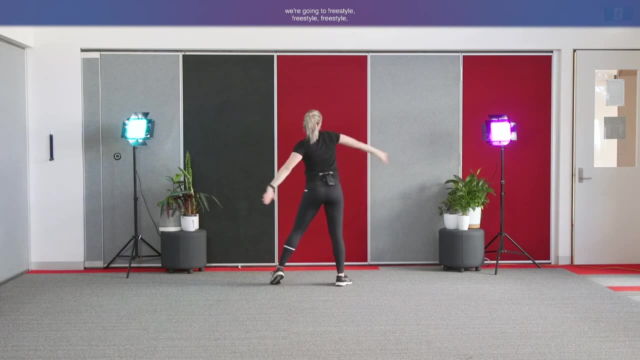 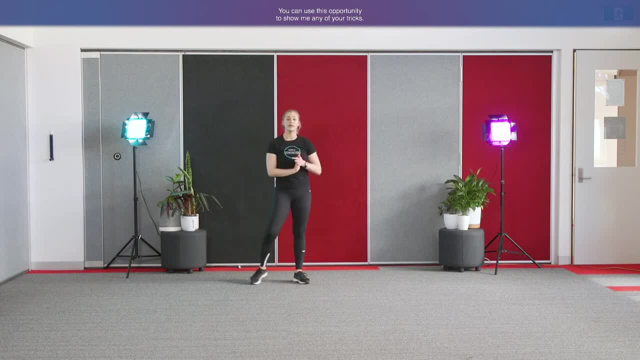 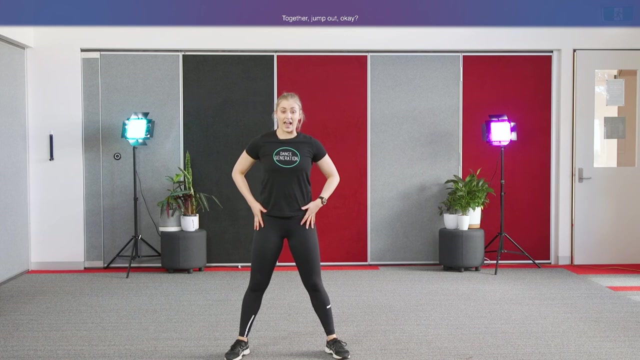 So you can do anything you like. You can use this opportunity to show me any of your tricks: splits, kicks, anything is awesome, But freestyling, freestyling, freestyling, turning around, and then we go five, six, seven together, jump out. Okay, That's how we're finishing. 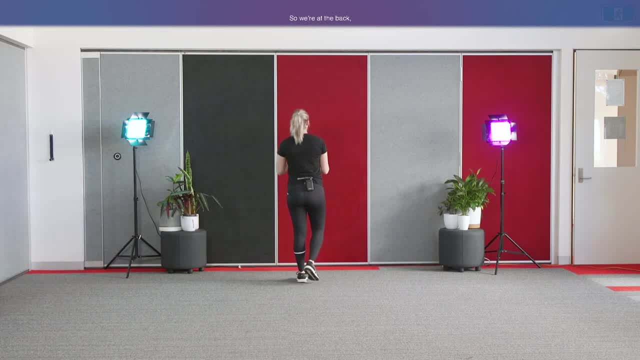 Okay, Okay, let's go through that one more time. so we're at the back and we go, freestyle, freestyle, freestyle, freestyle. i think it's maybe eight counts, it could be 16, but we'll see how we go when we've. 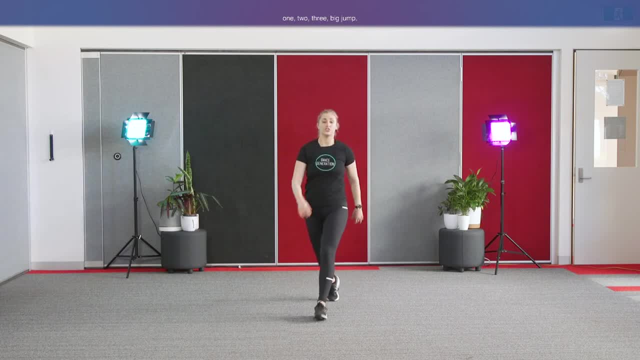 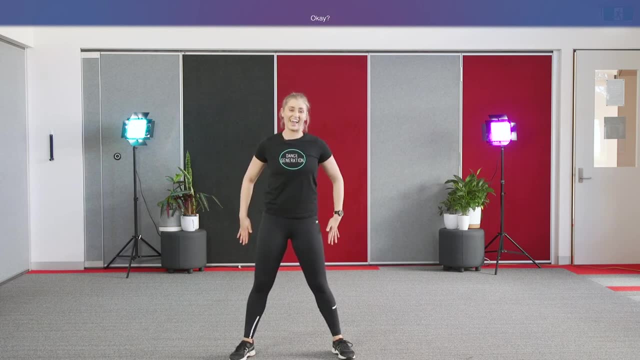 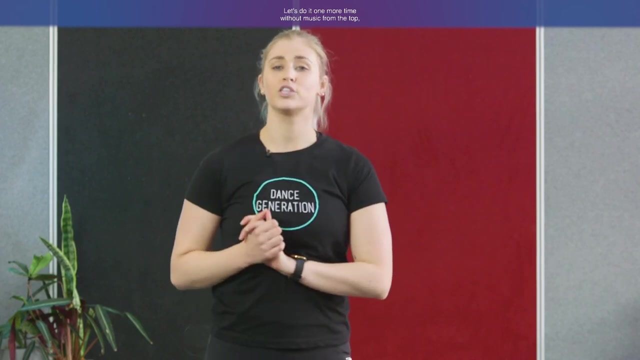 got the music and then we turn around one, two, three big jump. so that's a big jump, legs apart, and you're kind of kind of like hitting your thighs, okay, and that's it. that's it. it's fast, but it's fun. let's do it one more time without music from the top, adding in the freestyle and. 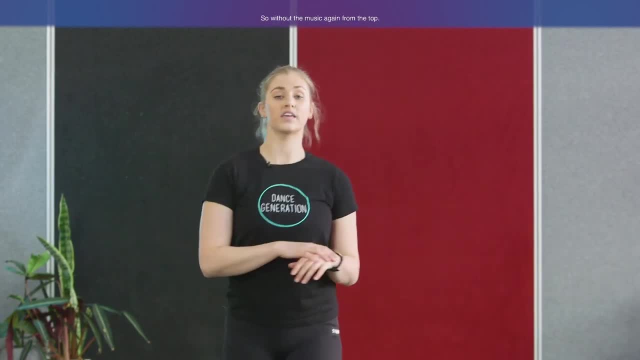 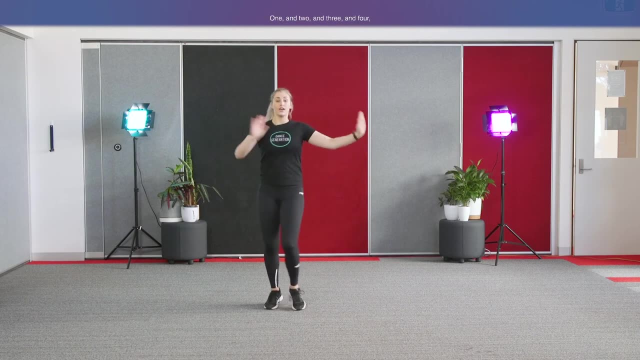 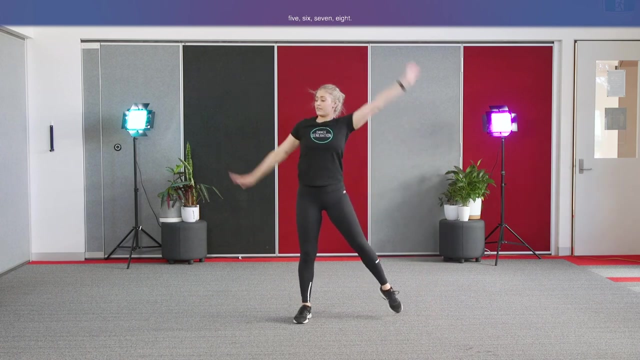 then we'll have a go with the music. okay, so, without the music again, from the top, hands on your hips, right knee popped, we go. five, six, seven, eight, one and two and three and four, five, six, seven, eight, one, two, three, four, five, six, seven, eight, one, two, three, four, five, six, seven, eight, one. 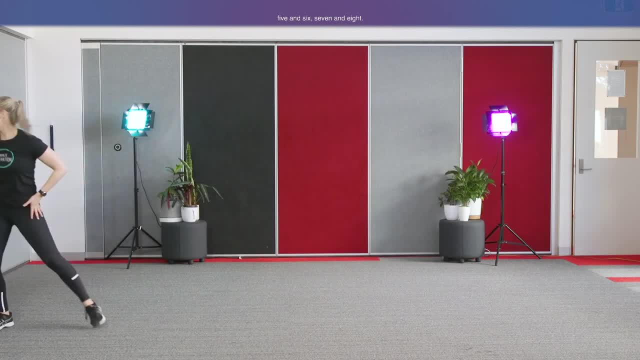 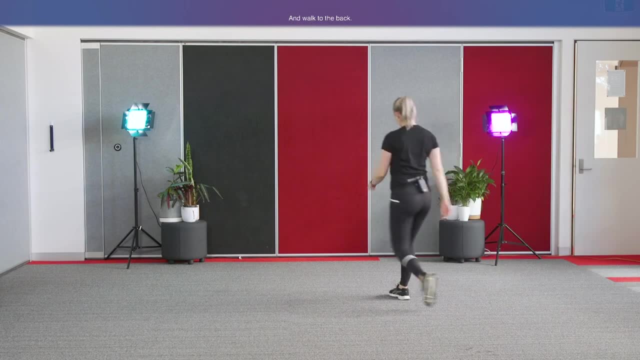 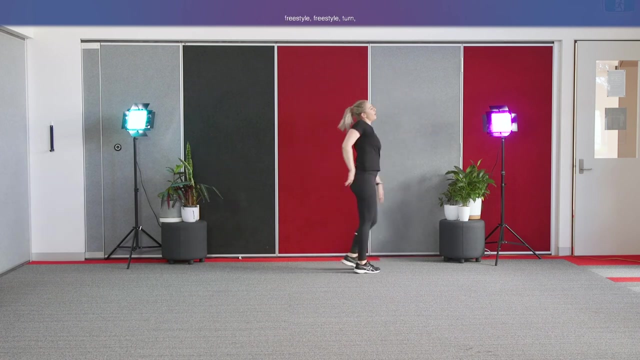 two, three, four, five and six, seven and eight. one and two, three, four, five, six, seven, eight, step, push and walk to the back from here, freestyle, freestyle, freestyle, freestyle, turn. and then, when the beat changes, we go: one, two, three, jump. okay, a lot of energy. let's do that again from the top. let's 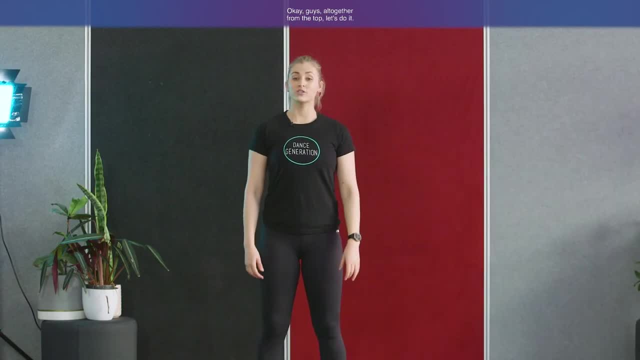 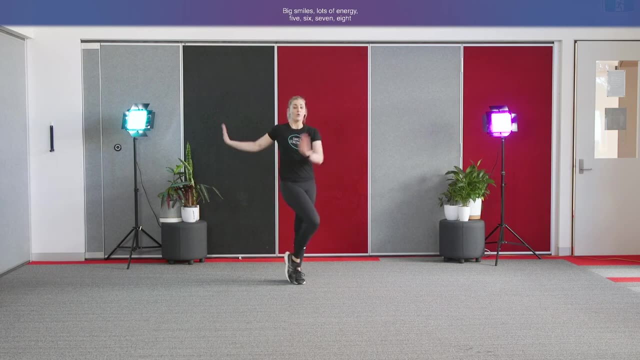 try it with the music all together. okay, guys, all together from the top, let's do it. we can do it. big smiles, lots of energy. five, six, seven, eight, one, two, three and four. five, six, seven, eight, one, two, three, four, five, six, seven, eight, one, two, three in and step up, step, step, jet and head one and two. 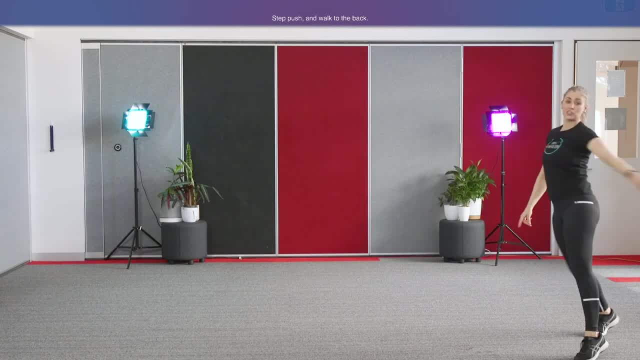 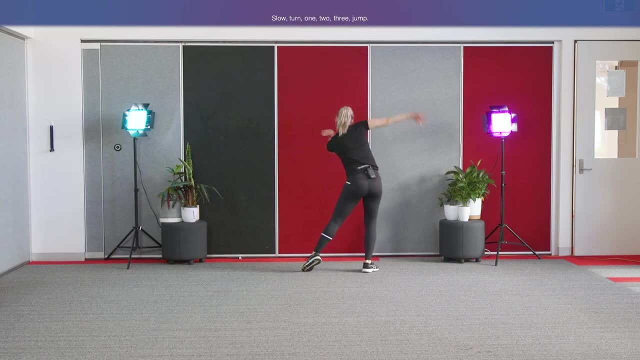 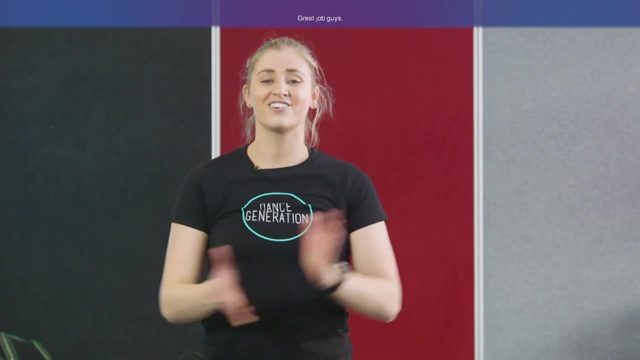 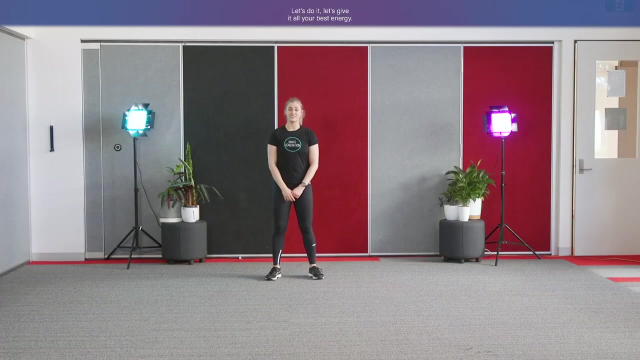 three, four, five, six, seven, eight, step, push and walk to the back and reach, slow, slow turn. one, two, three, jump. good, how did you guys go? great job guys. let's do it one more time from the top. okay guys, last time with the music, let's do it. let's give it all your best energy. five, six, five.